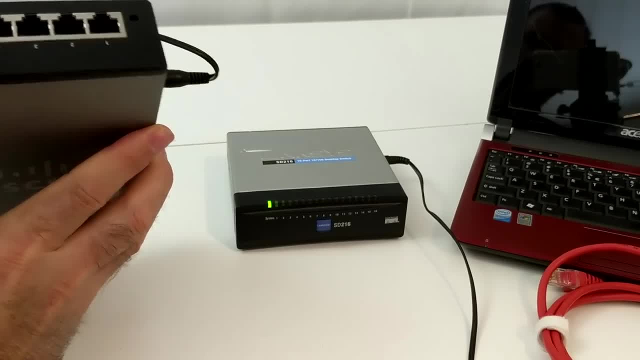 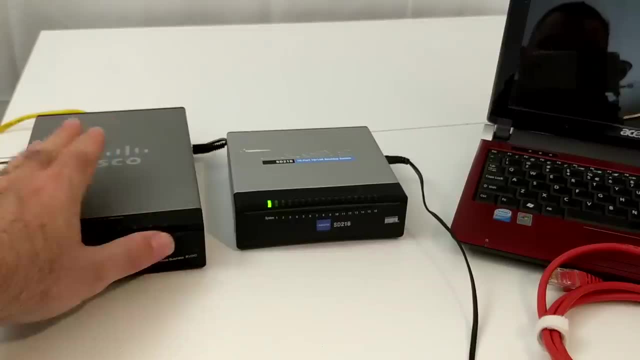 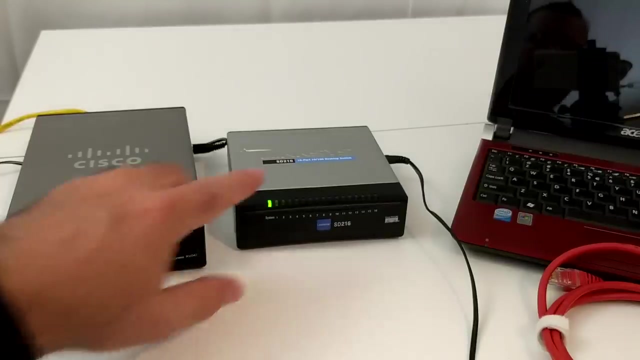 address and plug it into the router, and then what happens is it takes that one IP address and creates a subnet which allows the router to share that one interconnect internet connection with several different machines. But conversely, a switch is really just kind of like a port multiplier, All these. 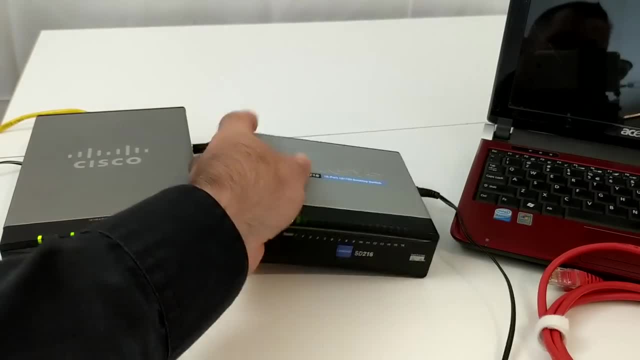 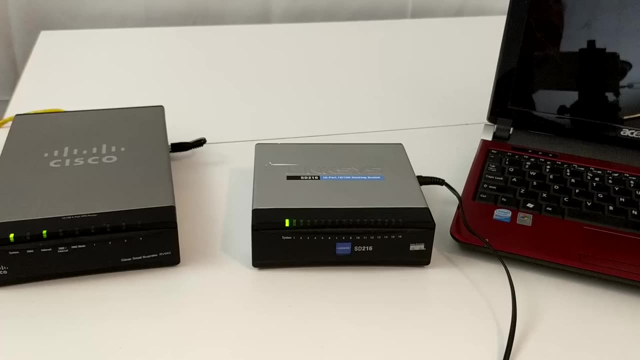 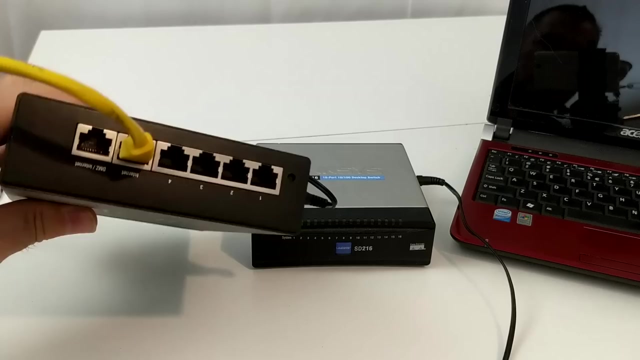 ports right here are the same. What it does is it takes a another handoff from a router and then creates a bunch of other network connections. But now this is where it gets a little blurry. A lot of today's routers, especially small office and home office, come with switch ports built in. 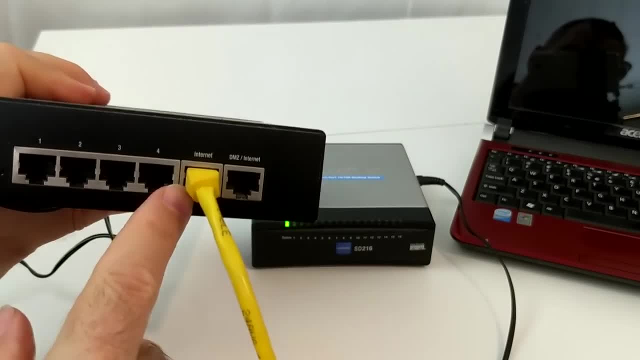 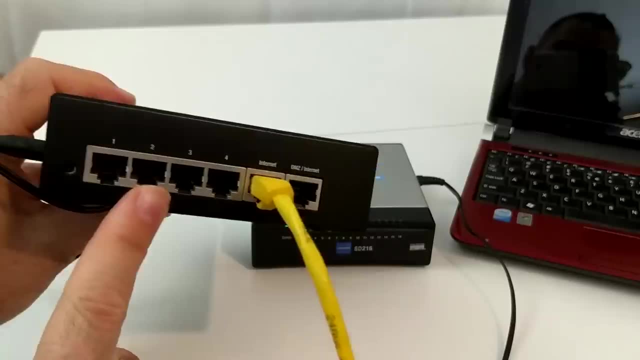 meaning that it's got a place for the network to go in, sometimes labeled wide area network or internet, but it's also got switch ports, meaning that it's both a router and a switch at the same time, However, unless you happen to be in a really small office, 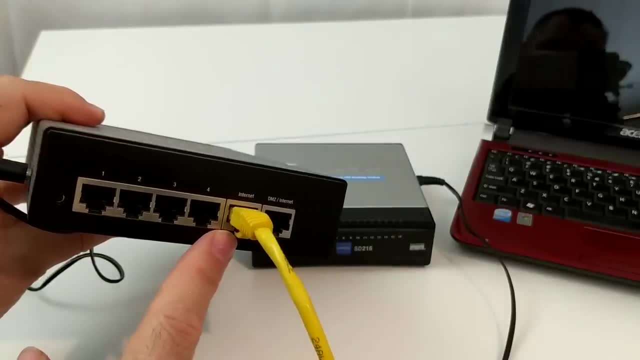 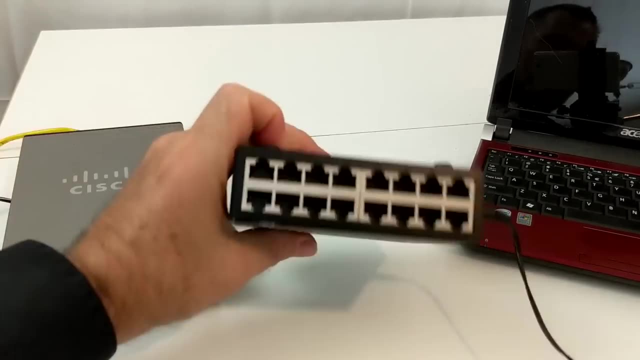 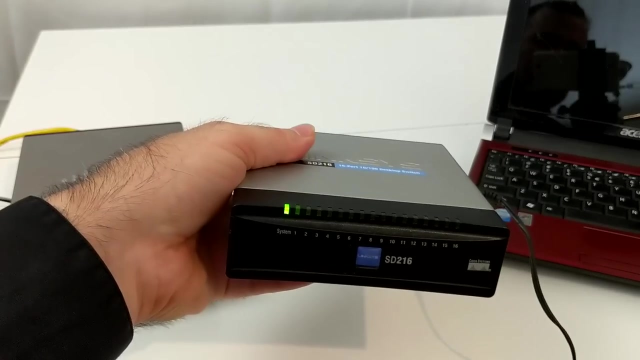 generally, you need more than four switch ports. You need more than four network devices connected to your router. That's where the switch comes in. The switch is like a outlet strip. It takes one connection and gives you a bunch of other ones, But there's no intelligence. I mean, there is such a thing as a smart 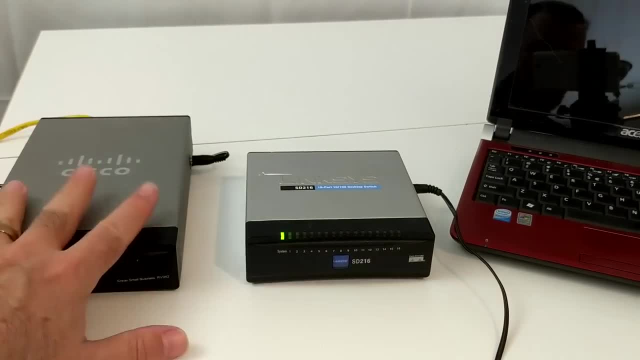 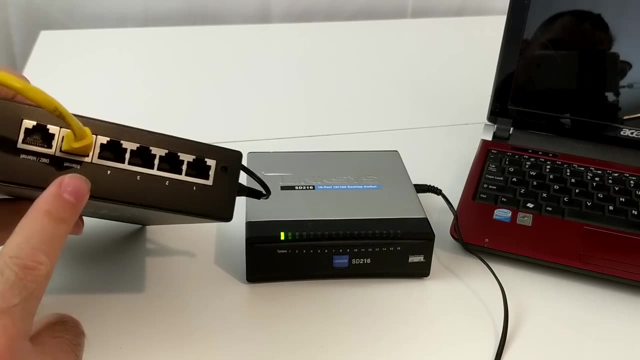 switch and in fact they even make switches that have routing capabilities For the purposes of this conversation. let's just stick with a dumb switch So I can take that internet connection that went into the router. take one of the switch ports, add another network cable and then connect. 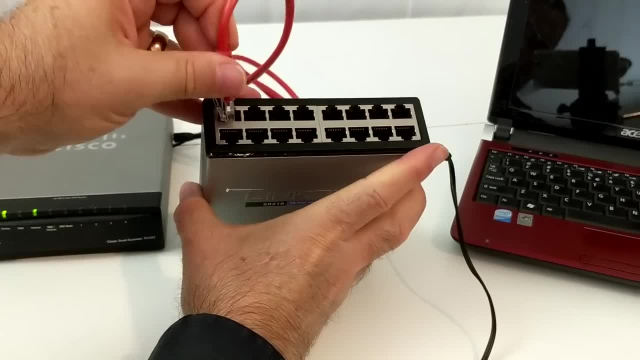 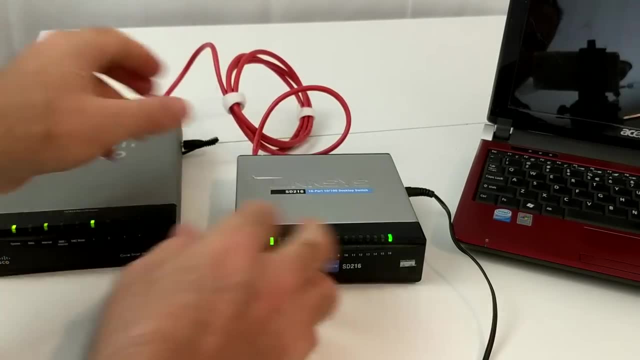 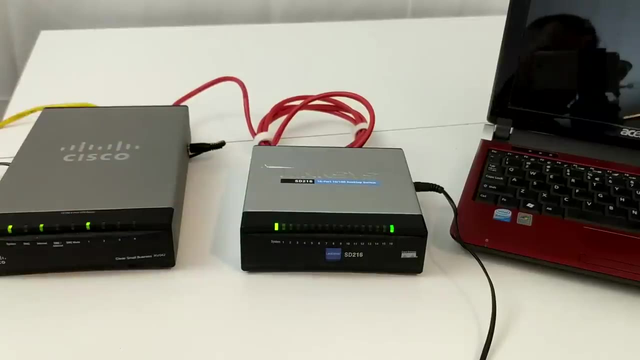 that to the switch, And now I have just taken what was originally four available switch ports on the router and just added another 15 ports to it. Alright, so I went from four to roughly 18 ports now, But the switch it's only job is just to. 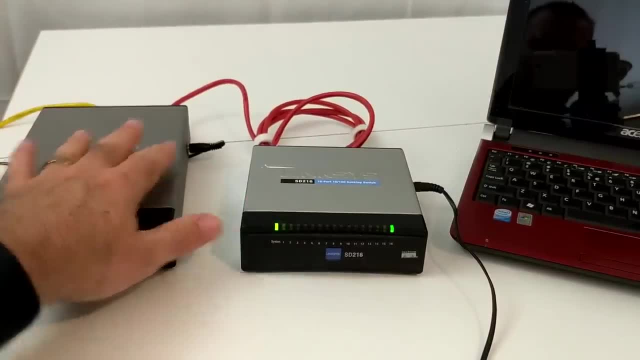 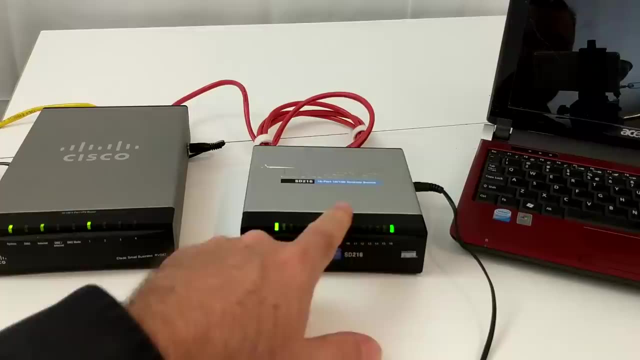 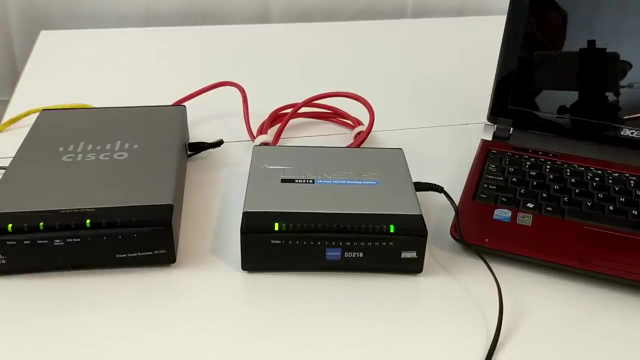 is just to is to take the packets that come from the router and forward them on to other network devices in the local area network. It can't make that translation between the local area network and the wide area network, the internet. Okay, so the router's job is to take the internet connection and provide a 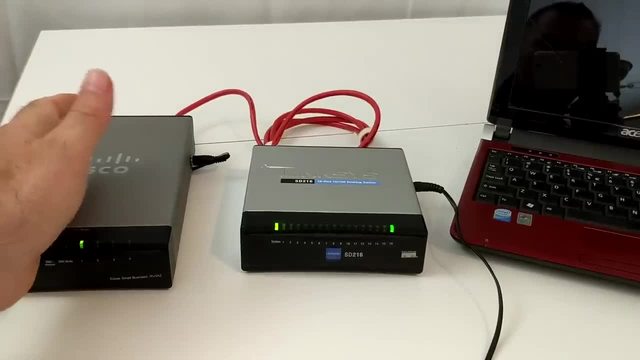 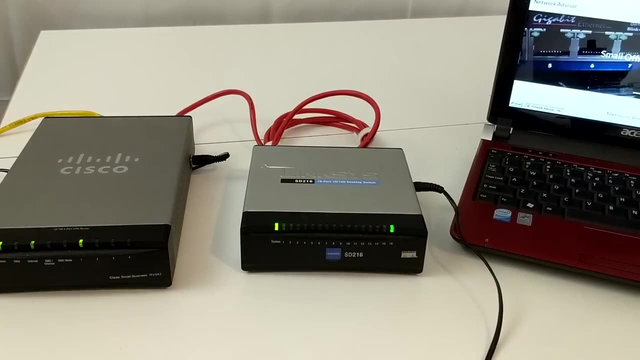 routing bridge between the outside world and the inside world, meaning all your local area network devices, computers and printers, and wireless access points. And then, finally, you take patch cords that are either connected directly between the computer and the network's switch or, in some cases, if you have a 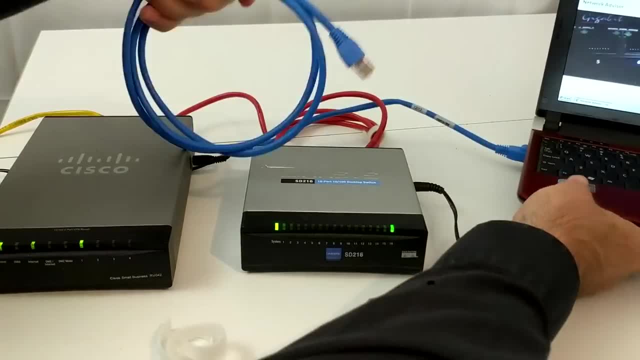 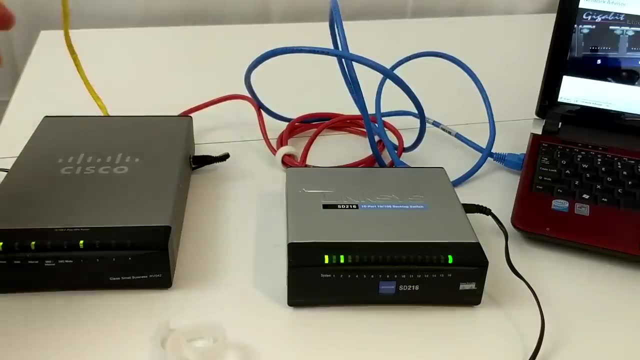 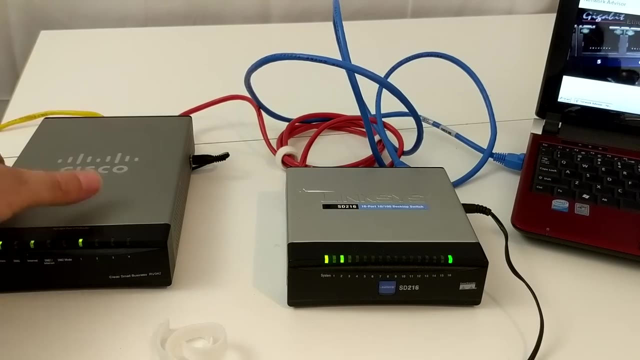 wiring system. they're actually going into a wall outlet which then goes to a patch panel which then goes to switch. So let's recap what happened here. We took an outside internet connection which was given to us probably from either a DSL modem or a cable modem or maybe even a T1, which is usually seen more in bigger 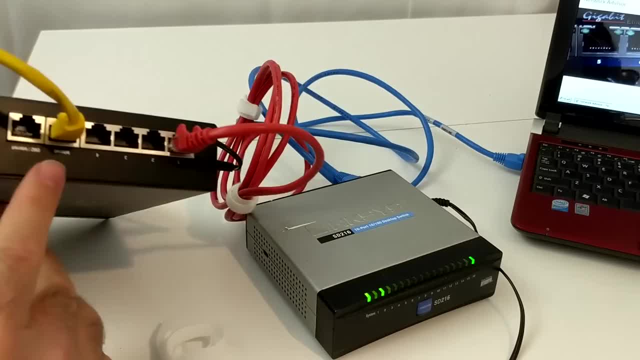 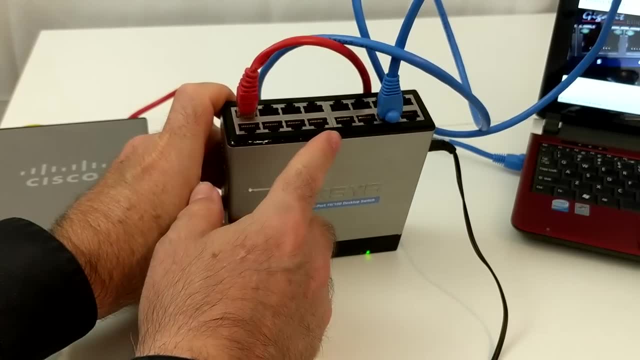 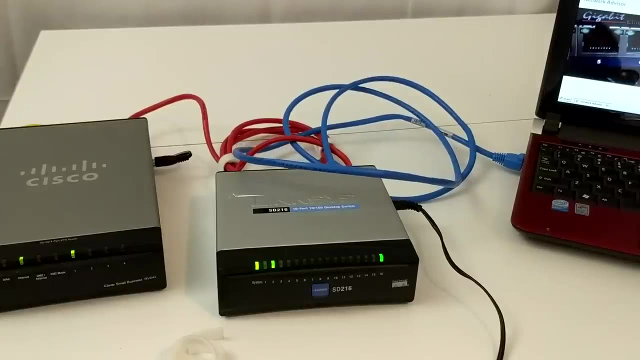 offices. We went into a router, we came out of the router's switch port and, in order for us to make more switch ports, we went into a 16 port switch and then out of that 16 port switch we went into a PC. So basically, the difference between 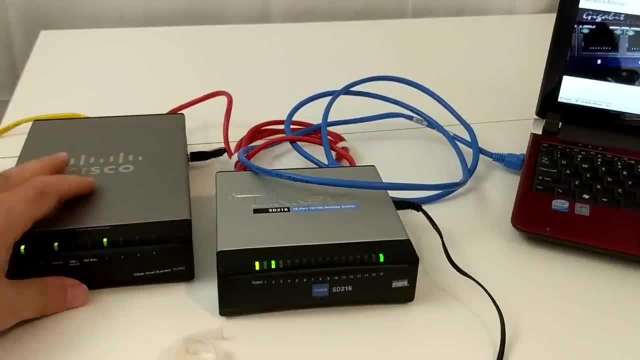 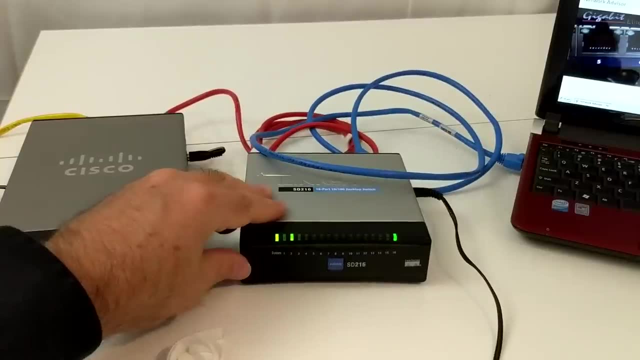 a switch and a router is that a router bridges an outside network with an internal network or an outside wide area network with an internal local area network. A switch really just provides additional ports within the same local area network. Hope that helps you out if you've. 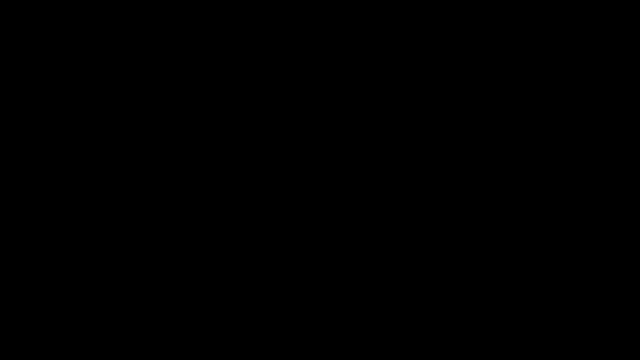 ever wondered about the difference. Thanks so much for watching. 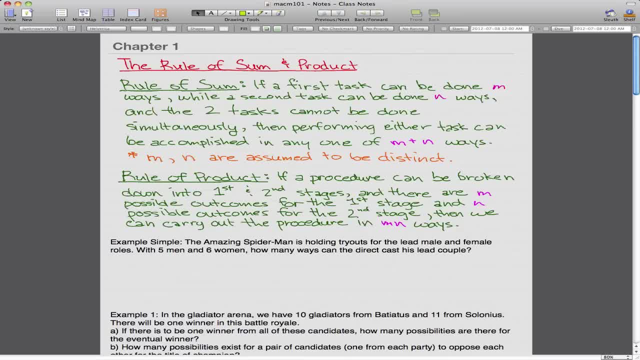 So we're finally gonna do the first series for discrete mathematics, and that's discrete mathematics 1. We already have discrete mathematics. 2. We started off at 2 first because my friend did that part and he's better at it than I am and I didn't really have time to do discrete. 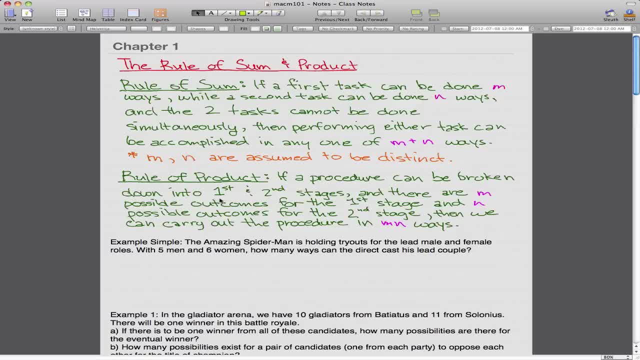 mathematics: 1. But here it is. First of all, discrete mathematics is a pain in the ass and I really don't like it. But I somehow managed to get a pretty good mark in class, so that's why I'm forced to do this. But I really don't want to. But I guess it might.